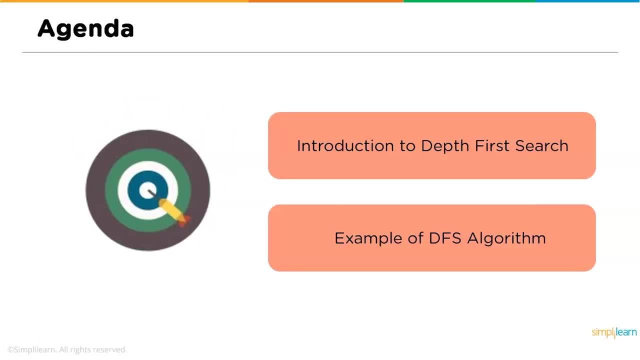 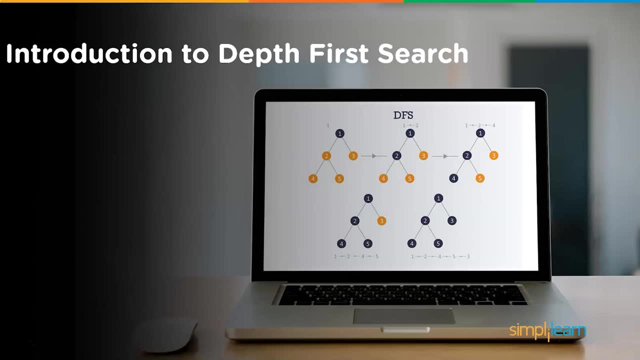 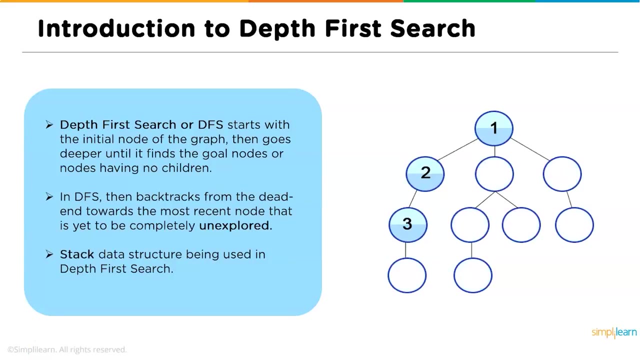 search, Followed by that we will look into an example for DFS algorithm. So I hope I made myself clear with the agenda. Now let's get started with the introduction to depth-first search. So what is a depth-first search? So, basically, a depth-first search is an algorithm for traversing or searching the tree or graph. 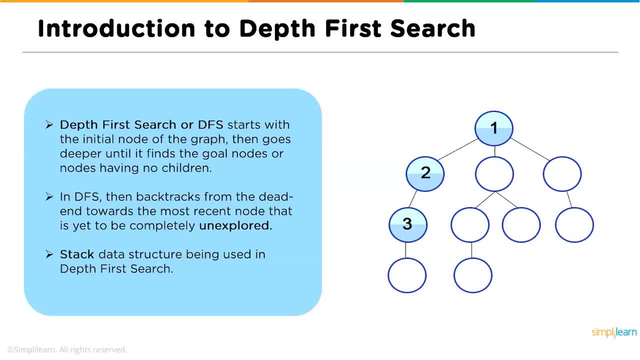 data structures. The algorithm starts at the root node, selecting some arbitrary node as the root node in case of graph, and explores as far as possible along each branch before backtracking. So DFS starts with the initial node of the graph, then goes deeper until it finds the goal nodes or the leaf nodes, or the nodes 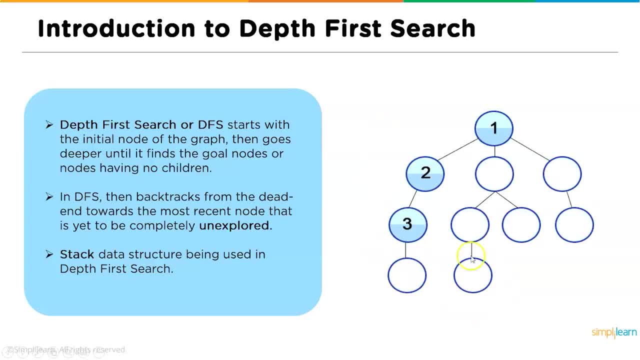 at the end of the graph. Here you can see 4 and 7 are the leaf nodes. So the depth-first search algorithm runs till the end of all the nodes, that is, 8,, 10,. all these are the leaf nodes or the last goal nodes. In DFS the backtracking starts once all the nodes. 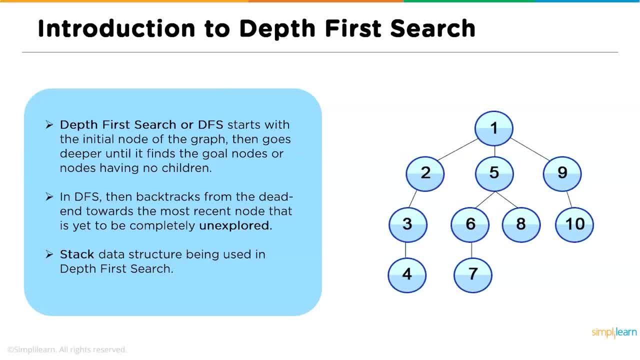 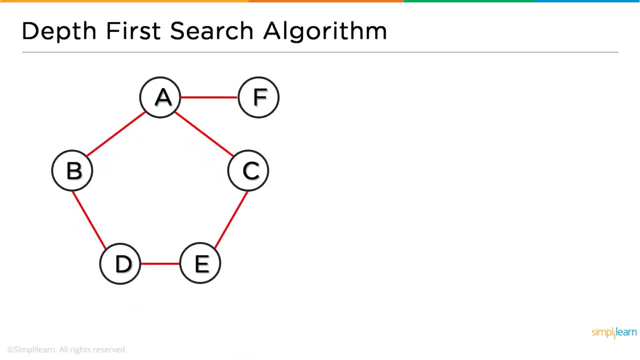 are explored, And the DFS algorithm uses stacked data structure for its traversal. Now, that was a brief introduction to the DFS algorithm. Now, for a better understanding, let's go through it. So here we have a graph data structure with elements A, B, C, D, E and F. So we will be 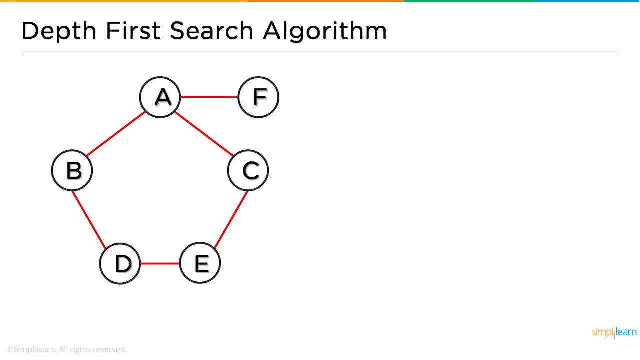 running the DFS algorithm and we will be traversing through all the nodes of this particular graph And the traversal will be recorded using a stacked data structure And we have two different colors which will be used to indicate the element's color. So the black color is for the nodes which are not visited yet And the blue color will 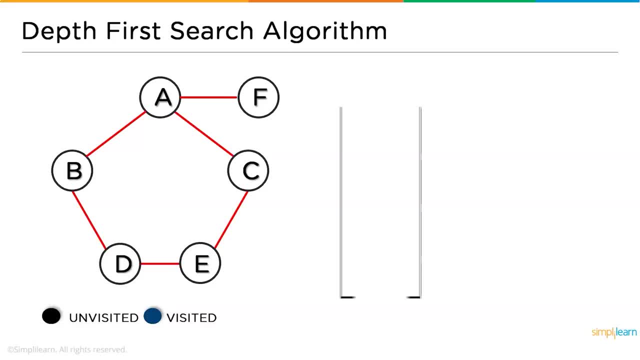 indicate the nodes which have been traversed already. Now, this is the state data structure which we will be using for the traversal, And we have another part which declares or which gives out the output of thesto traversal of nodes of this particular graph. 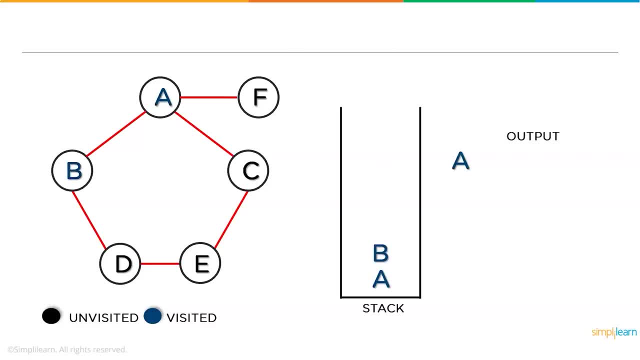 Now we will begin with the first one, that is A- No. followed by that we will move ahead to B. After B we will go through D. the after D we will have E. Next we will get to A. the next one is code E, Then after D we have E, Then after D we will move ahead to B. Then